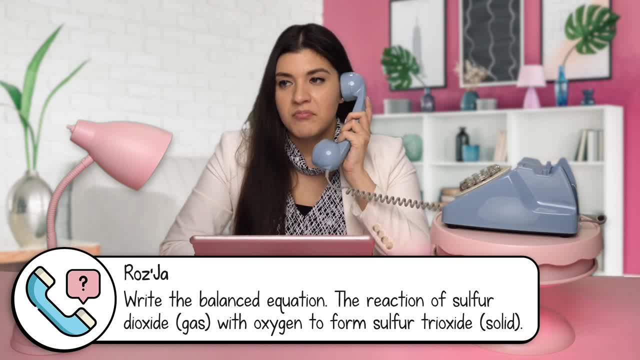 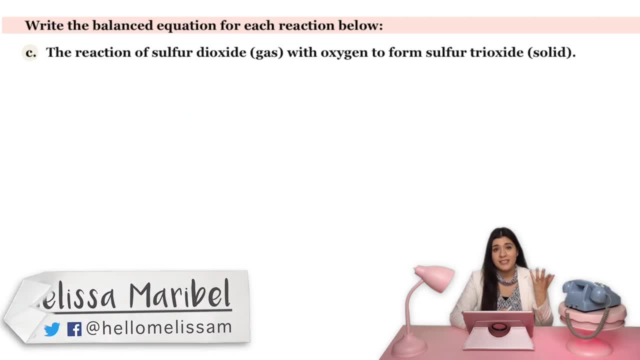 with oxygen to form sulfur trioxide solid. Okay, Here it is. Let's go over that. So for questions like these, where they're pretty word problems and we're trying to translate and see what they mean, the best thing is just to identify key words here. So, first things, first of course. they're telling us. 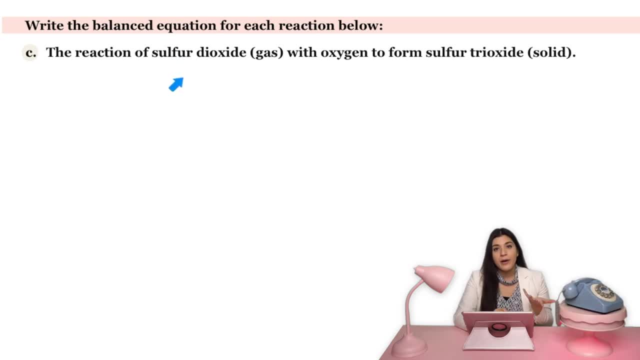 the specific elements and compounds that are involved in this reaction. So the first thing that I want to identify right now is: just what is sulfur dioxide? So what is the chemical formula for it? So, for sulfur dioxide, let's just start off with: is this an ionic compound? 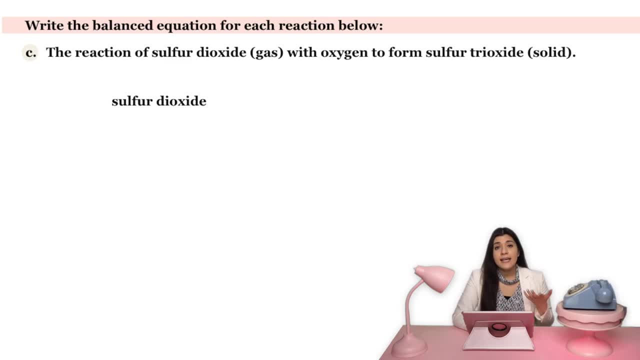 meaning? is it a metal and a non-metal, Right? Or is this a covalent compound, meaning it consists of two non-metals? So how I instantly know it's covalent is just by the prefix, The fact that this has the word di there. 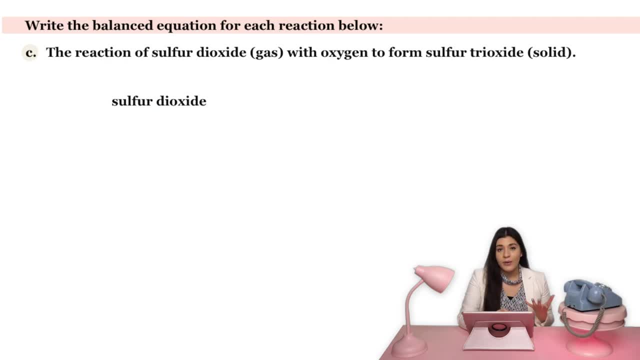 that prefix, then I know that it has to be a covalent compound, meaning I don't have to balance any of the charges whatsoever. Okay, So in this case it's really just sulfur. so S Di refers to two. So for a covalent compound, that's always telling us that prefix. 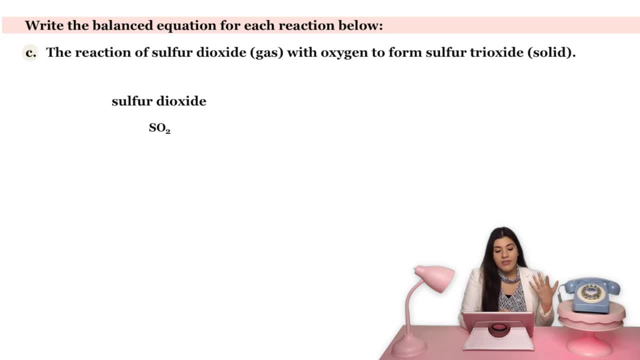 is always telling you how many of that specific element there are in this question. Okay, So in this case it's dioxide, so there are two oxygen, So that's O2.. And then remember, anything that ends in "-ide just means that there's only one element there. There are. 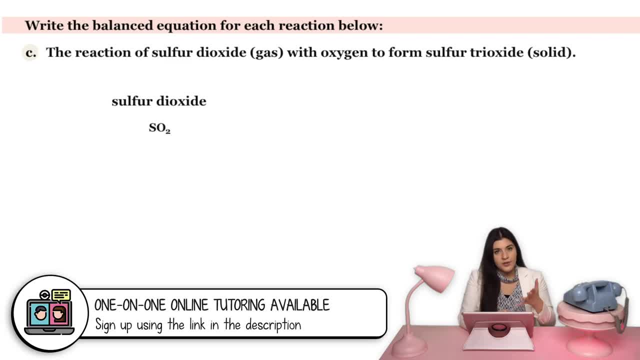 some exceptions, for some polyatomic ions, but for this type of question, that just means that it's just oxygen. Okay, So this is SO2.. That's what it's referred to as sulfur dioxide. Continuing on This now says with oxygen. Be aware of this. Sure, it says oxygen and you would think. 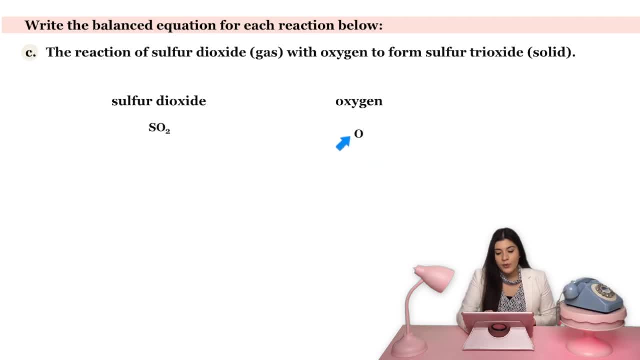 okay, it's singular, It's just one oxygen. It's not going to be plural, That would be wrong. So oxygen doesn't exist on its own. Okay, This is a type of diatomic molecule. Diatomic molecules are really just molecules that exist in pairs, So instead of O, it's 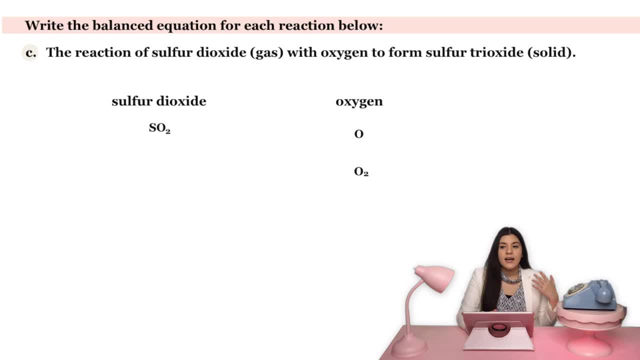 going to be O2.. And then a lot of these are like, let's say, hydrogen is a typical type. for it It's not going to be any sort of halogen, And especially because this is a type of gas as well. So for oxygen it's not just going to be O, It's going to be O2, and that's definitely. 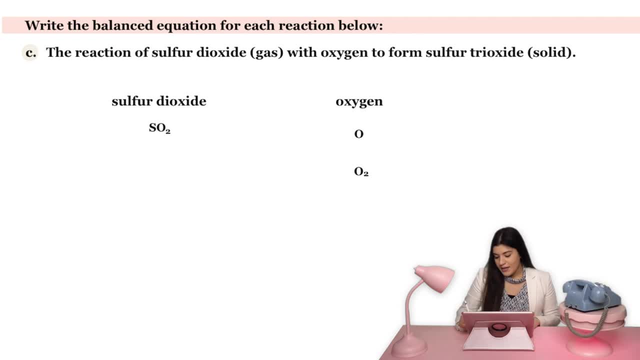 something you need to know. Okay, So they're trying to trick you there. And then next it says to form sulfur trioxide. So I know, okay, well, this is sulfur trioxide. Once again, is this a ionic compound or is this covalent, The fact that there is a prefix? 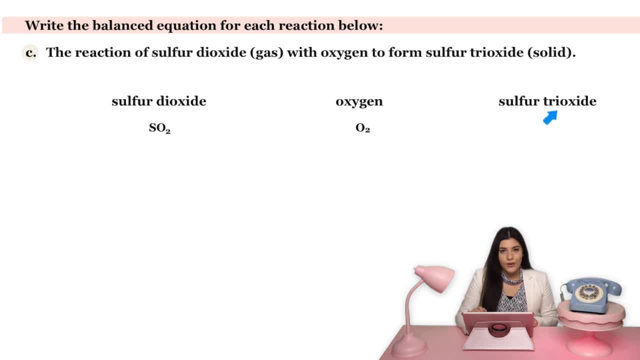 here of tri tells me that, okay, this is a ionic compound. Okay. It tells me that, okay, it has to be covalent. I don't have to balance any charges whatsoever, So all I have to do is write this out. where I know, sulfur is S, Tri is the prefix for: 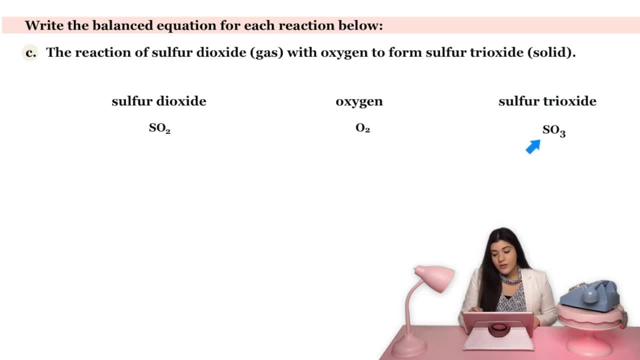 three. So I know that there are three oxygens, So that's why it's SO3.. Next part of this: now that we identified all of the different compounds that we're working with here in the types, then I want to identify what are my reactants and what. 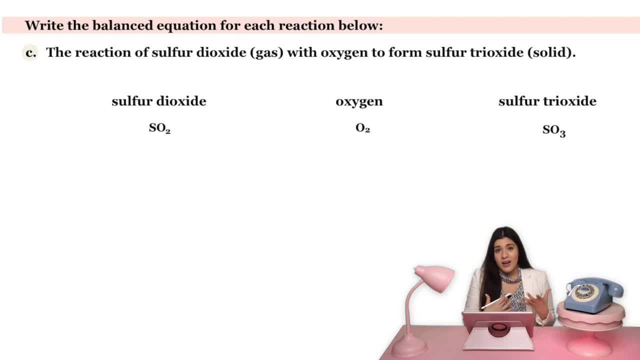 are my products. I need to identify major keywords here. So one of the major keywords here is the fact that it says with. So that with is telling me okay. well, I know that that means plus Okay. So whenever it says like, oh, sulfur. 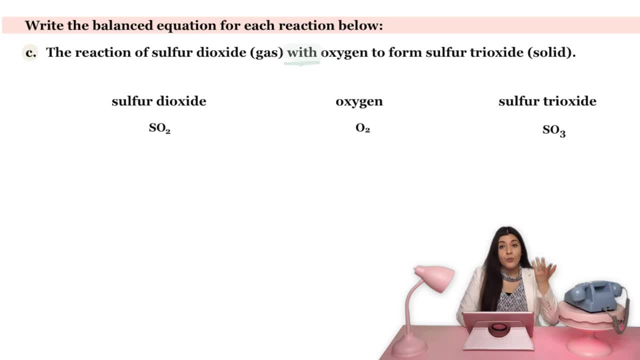 trioxide and oxygen, or with oxygen. that means we're adding those together. So the reaction of both of these, this says sulfur dioxide with oxygen. I know that both of these are going to be my reactants. Next, this states to form: 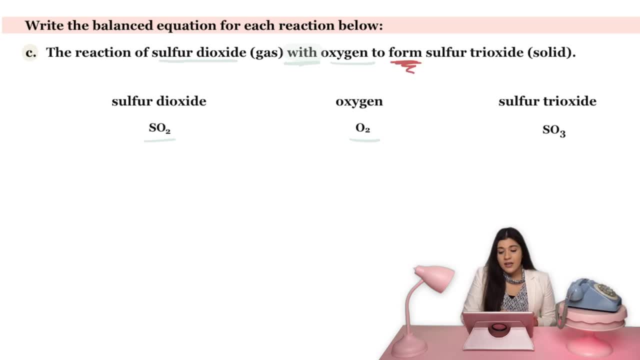 If something is being formed, that means it's going to be your product, So I know that sulfur trioxide is now my product. All right, So that's the main thing here is that I'm just looking at. okay, what are the keywords, and and with, or sometimes it could even say sulfur. 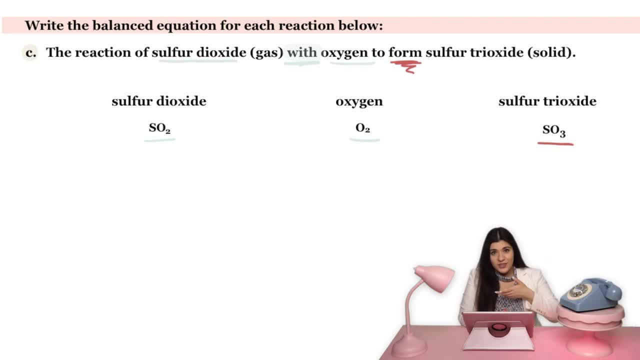 dioxide reacts with oxygen, So that saying reacts also tells me it's a reactant. Now that I have identified those two, I can build this and put this together. So I know that these two are my reactants and it forms our sulfur trioxide. 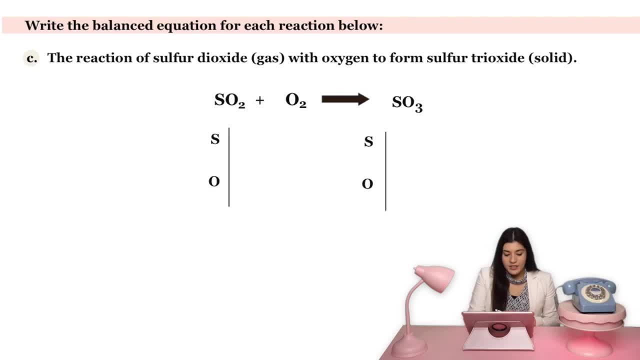 Next, we want to balance this out. What we're going to do is figure out how many of each elements there is on either side. So in this case there's only one, sulfur. We'll count how many oxygens there are. So here we have two, plus this additional two because it is 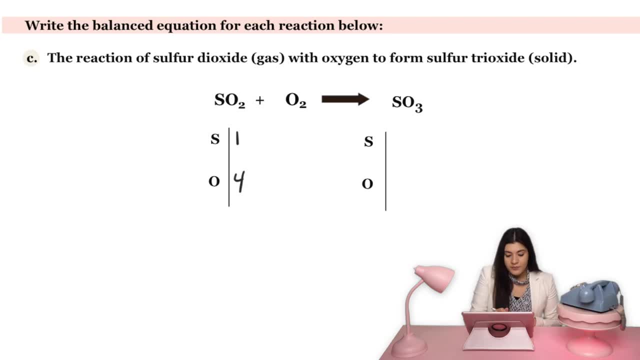 on the reactant side. So two plus two would give us four. I'll look at the other side here, So the product side. there's only one sulfur, And then, due to the subscript of three, there are three oxygens. Okay, 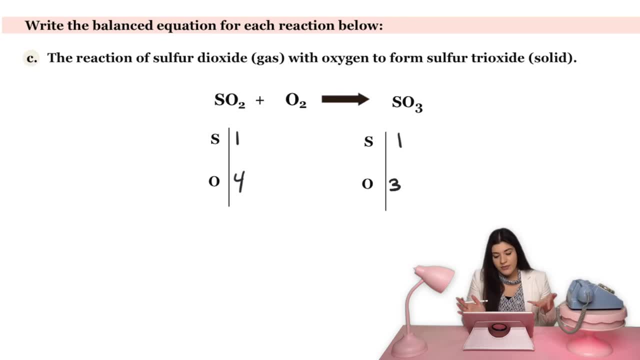 So what I will do now- because sulfur is balanced, it's fine, It's the oxygens that aren't What I want to do. let's say I'll put a two and I'm going to distribute this two and recount everything up. Okay, So if I recount everything, this now is two sulfurs and this is two times. 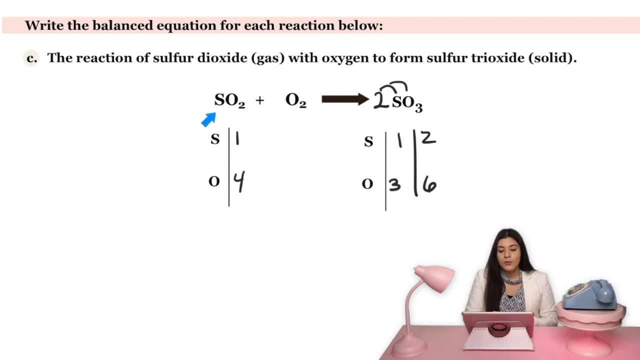 three, So six. Now I'm trying to figure out what am I going to do. What am I going to place to make the amount of oxygens on the reactant side be six? So, instead of doing anything here with our oxygens, because the fact that sulfur has 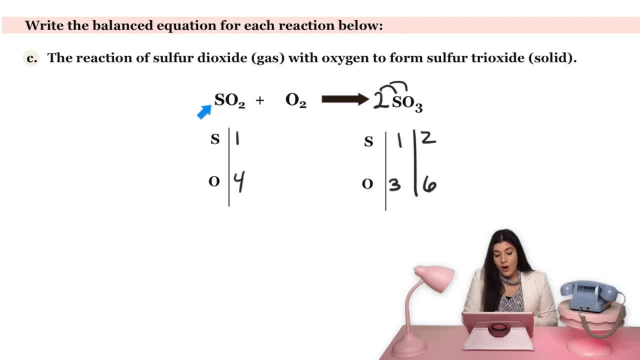 two. now that means we must place a two in front of SO2.. So I have to have a two here. I'll distribute and recount everything on the reactant side. So I now have two sulfurs and double checking here. this is two times two, giving us four, Four plus this additional. 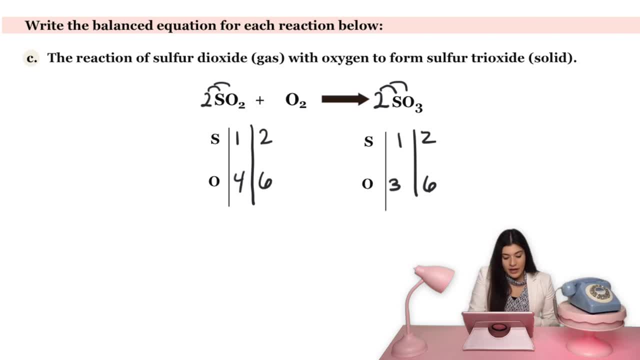 two would give us six. So now everything is balanced so far. So, now that we have this balanced, the next thing is just identifying all of our different states. So, luckily, this question told you. So it told you that sulfur dioxide is a type 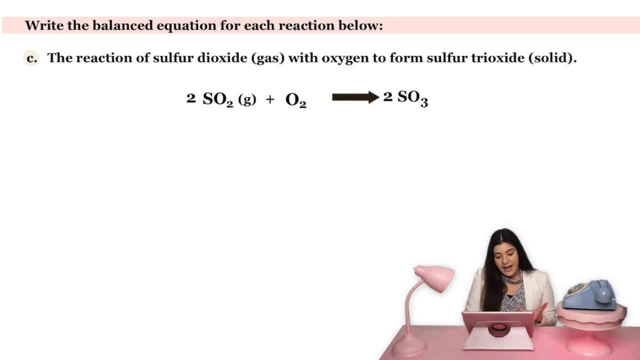 of gas, So I know that that's how I'm going to label it. Next, it is known that diatomic molecules tend to be gases, So oxygen or hydrogen or some sort of halogen. those are types of gases, So this is going to be a gas. And then, lastly, this tells you that sulfur trioxide 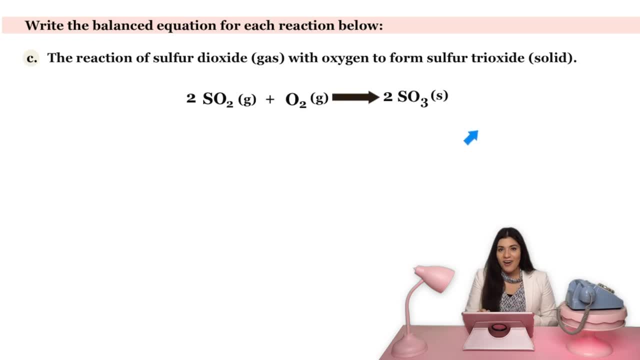 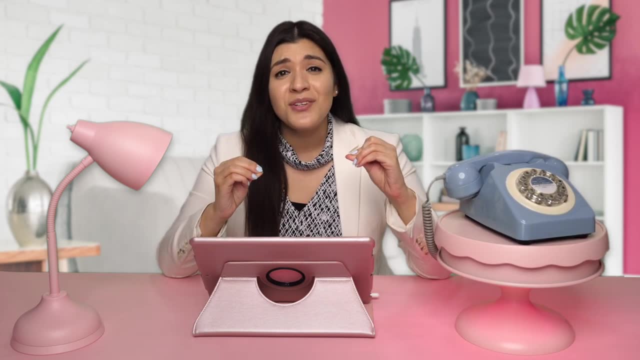 is a type of solid And this is how we get our final result. This question is a common quiz and exam question, So make sure to lock that down and know how to do this. And if you feel like you know what, I don't know what I'm doing in chemistry.